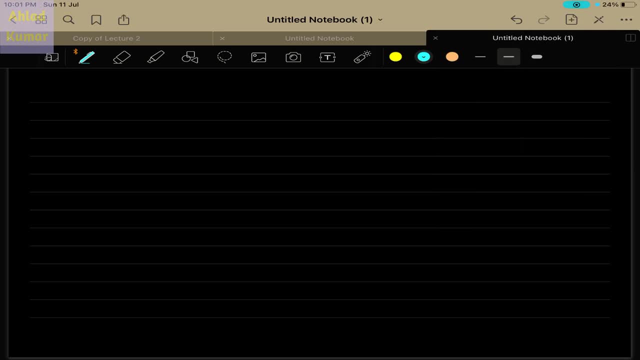 So in the last lecture we discussed the need for converting the sentences into the vectors, And one of the reasons for that was like how to you know feed these sentences into the existing machine learning architectures which actually require inputs in the form of numerical data? So one of the reasons was that, And the second important reason, other than this, was how to you know come up with these numerical data which are present in the vector. In fact, 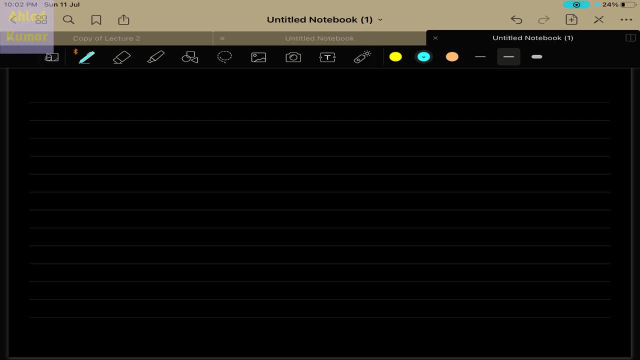 it captures or encapsulates the semantic relationship among the sentences. And that was another key takeaway point from the last lecture discussion. And I again repeat that we want to select the numerical- you know- values within these vectors in such a way that it has to semantically capture the significance of the sentences. So now today, we will discuss some techniques which actually convert. 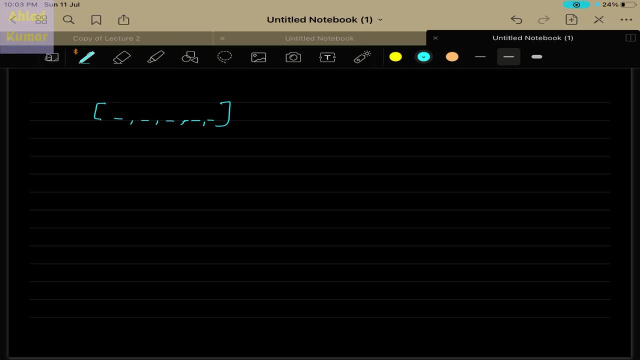 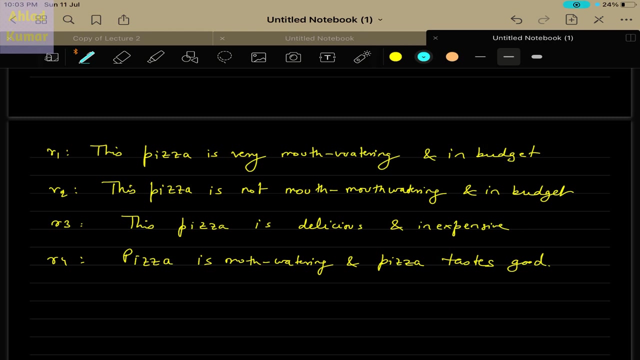 sentences or words in the vector format, And the very first algorithm that actually is used for this purpose is bag of words, which we also call as BOW. in short, In order to understand the concept of bag of words, I have here an example which actually contains four reviews for a particular, you know, pizza hut company. So these reviews are, you know, as follows: that the first review actually says that the pizza is very mouthwatering and in budget. 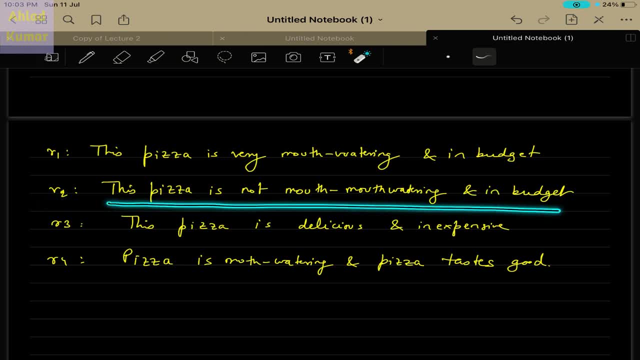 The second review says that this pizza is not mouthwatering and in budget. And the third review says that this pizza is delicious and inexpensive. And the fourth one says that the pizza is mouthwatering and pizza tastes good. So we have to see that. how to, you know, convert these reviews, which are, you know, given over here, into the form of vector so that we can use, you know, machine learning algorithms to learn the essence of these you know reviews? So these reviews are also basically called as BOW. 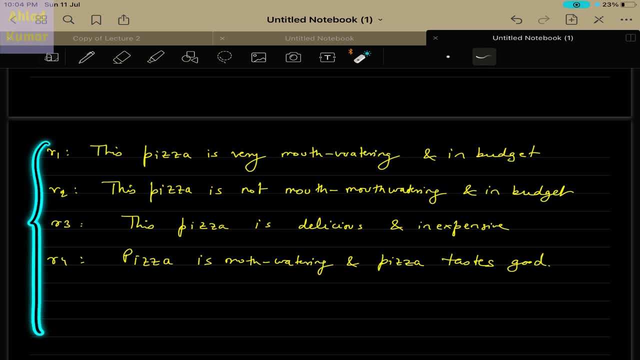 So these reviews are also basically called as documents And in the area of natural language processing, these individual, basically reviews are also called as documents. So we call these also as documents And the collection of these documents, that is, these individual documents that you have, you know, these R1, R2, R3, though we are writing it as reviews, they are documents, But collection of these documents is also called as corpus in the area of natural language processing. 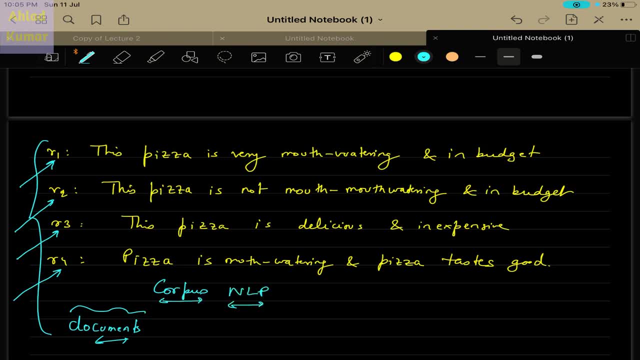 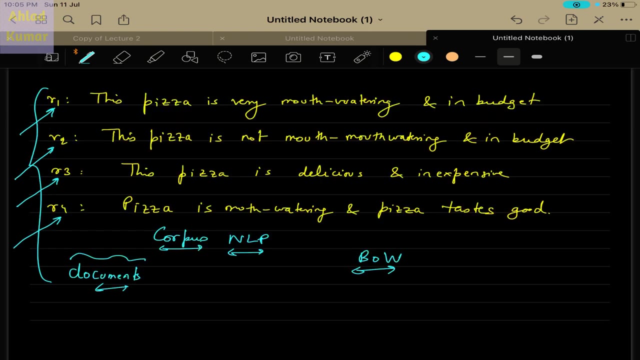 So we will see, you know how bag of words will be able to, you know, convert these documents or reviews into the form of vector which actually will be used for feeding into the machine learning architectures. So, in order to convert these reviews into a form of vector, there are actually two steps. So the first step is basically to construct a dictionary. So the dictionary is basically, we are representing it by a set V. 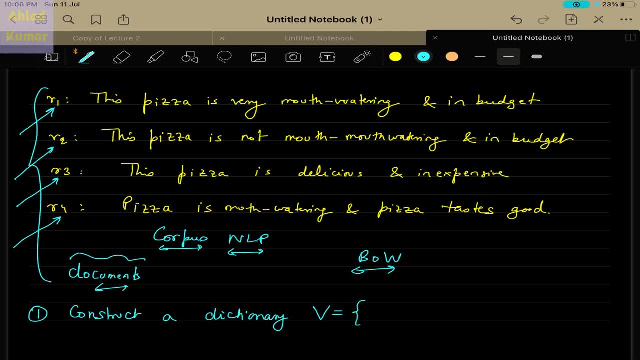 Which actually contains all the words that are present in the corpus that we are actually considering. Or maybe you can take the complete dictionary of English words. If we restrict ourselves to the words which are appearing in the complete corpus that we are looking here, then you know, dictionary will be, you know, a set of all the words. like you know, this pizza is very mouthwatering. 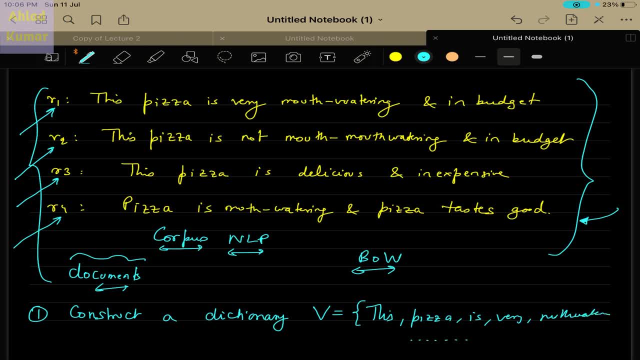 Like that. You will, you know, put all these individual words, all these individual words, And if they are repeating, you keep. you have to keep only a single word. And then you know, form a set of that word And you call that set as V. The dimension of this will be, you know, 1 cross D, You can say that And you know where D is basically the total number of words that you have in the dictionary. 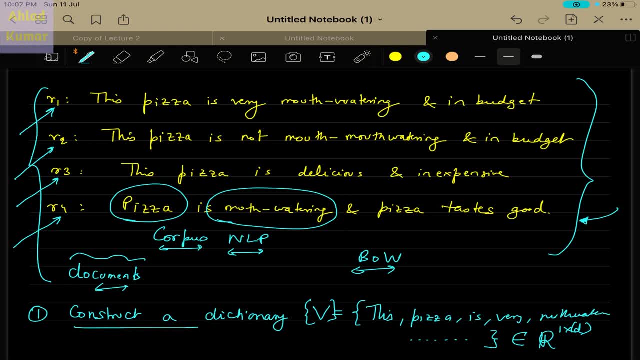 So the important thing is, first of all, you have to construct a dictionary, which we are calling as V. So all the elements of this set are basically the words that you have in the corpus which you are considering for the task of natural language processing. 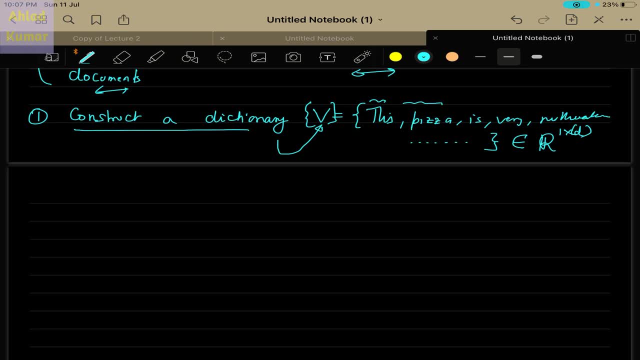 The second step, basically, is you know to form a vector. So let us say, if you want to, you know, convert the review 1 in the form of vector that will be, you know, given by V1.. For review 2, it will be V2.. For review 3, it will be V3. And for review 4, it will be V4. So all these will be the vector that will be formed using the algorithm which we are discussing now. 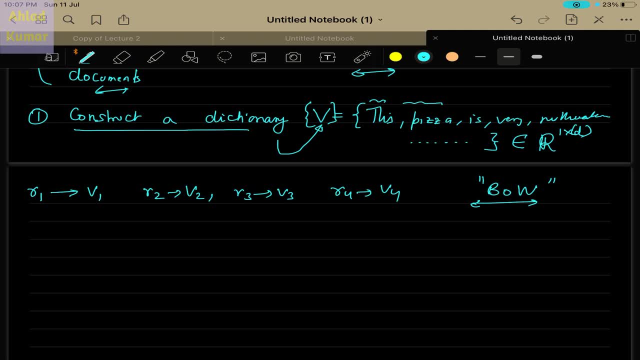 This is bag of words. So, using this bag of words, we will actually convert these reviews into the form of vectors. So, in order to form a vector V1, what you will do is you will first of all create a one-dimensional vector of size D, 1 cross D, where D are the total number of words that are present in the corpus. 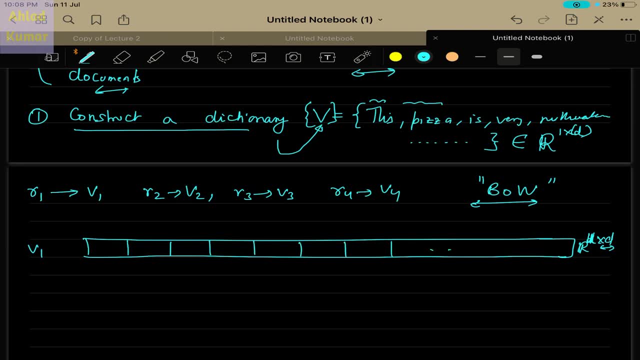 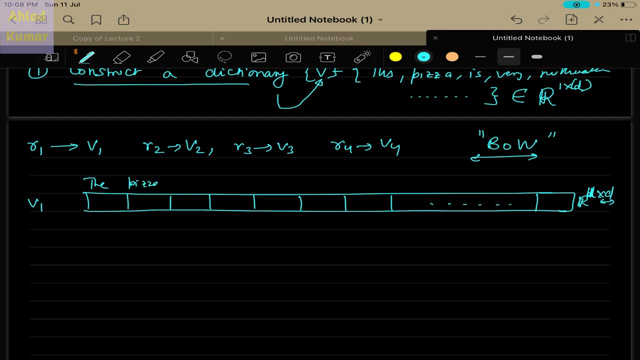 And what you do is you know you will create something like this. So this dimension is 1 cross D And here you can write the you know. for your understanding, you can write the words which are there. That is, the pizza is very mouth-watering and in budget. 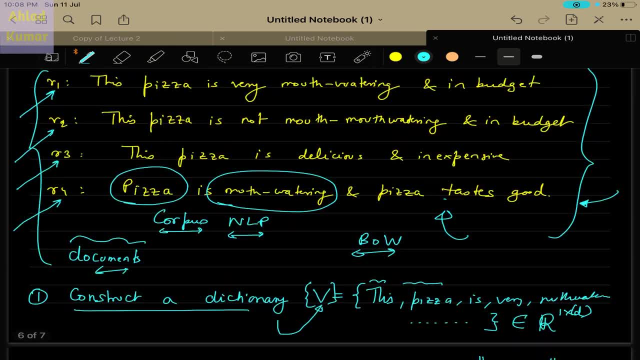 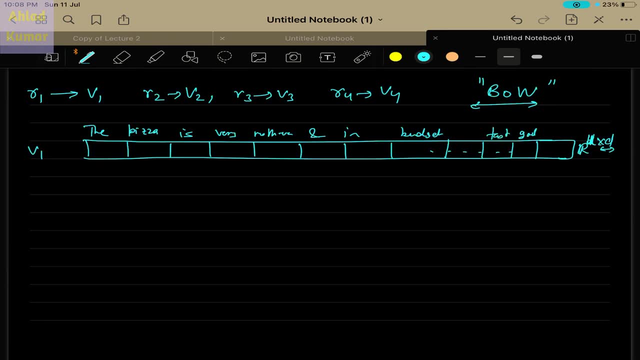 And you have other words also which are, like you know, taste good, inexpensive. So they will be, you know, here like taste good. So what you have to do now is you have to see like which words are actually appearing in the review and you have to keep the corresponding number in this particular vector. 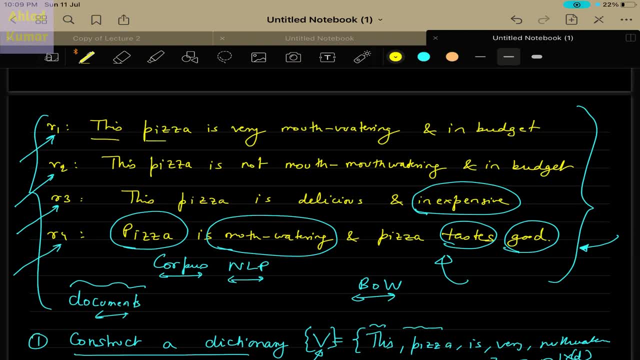 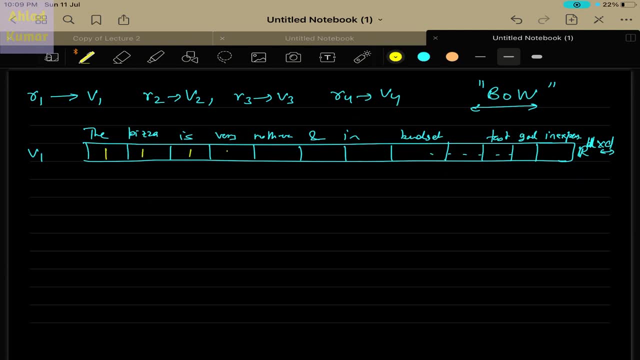 So, for example, in the first review you have this: pizza is very mouth-watering and in budget, So all these words are actually appearing. So we will put 1, 1,, 1, 1,, 1,, 1, and 1, and 1 here. So all these you know words will have 1.. 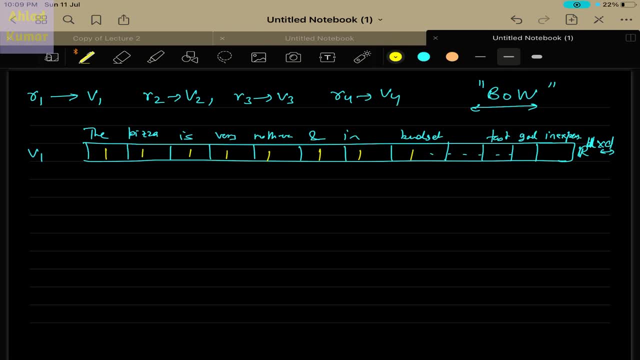 And the others which are not there, and other words which are not there and are still in the corpus, will be given 0s. So this is basically the vector representation V1 for the first review. Similarly, you can make the vector representation for the second review, which is V2, in the same fashion. 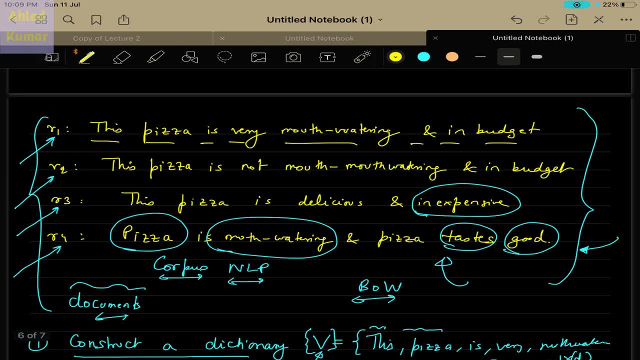 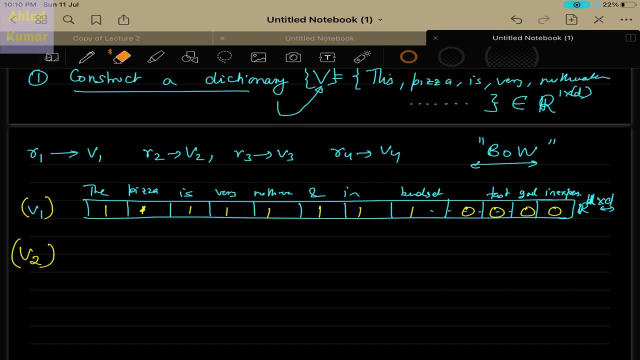 But note that in some situations where the words are actually repeating twice, for example here, the pizza is actually repeating twice: One is here and another one is here. So what you can do is you can replace this 1 in that particular representation by 2.. 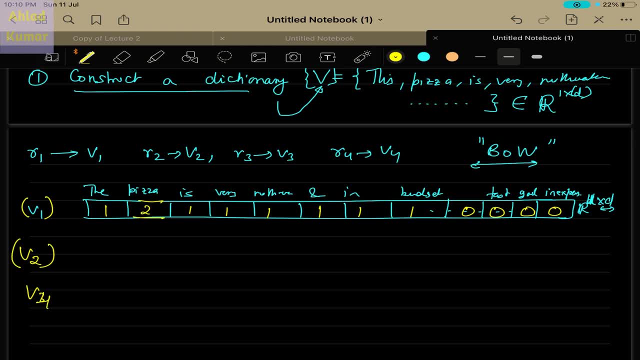 So when you write vector representation for V4, the corresponding component pizza here will have a value of 2.. So here it is still 1, just to avoid confusion. So in review 4, the corresponding vector representation having pizza as one of the elements, the value of that will now be 2.. 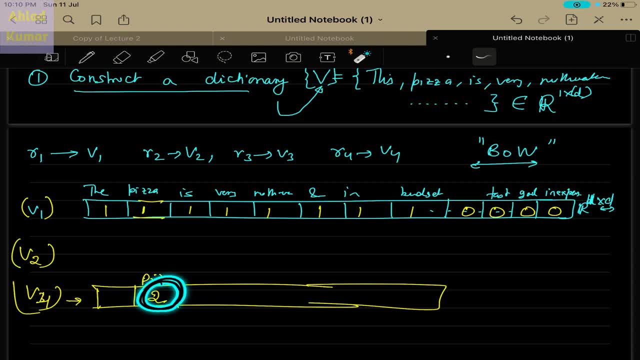 And the word pizza is now a character form of 1.. And the sole reason for that is because pizza is actually happening two times in the in the review. So what actually these elements in the array represent is the frequency of the word that is appearing in the review. 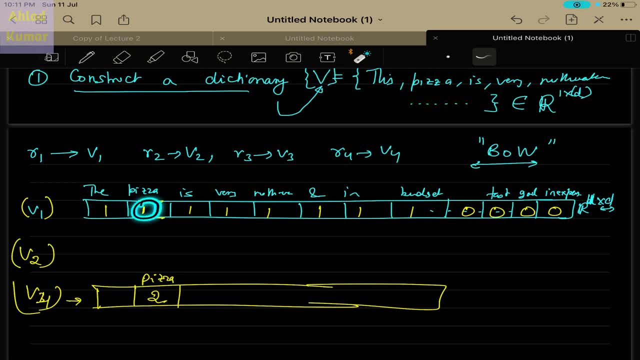 So if the word is appearing single time you can write it once, and if the word is appearing multiple times, and depending upon the number of times it is appearing, you have to write that count here. So it's a frequency of appearance. that is for that particular review. 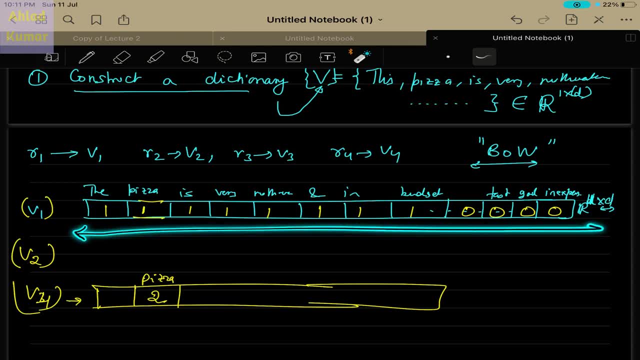 So now, In this way actually, you can represent the vector representation for the particular review. So this particular way of representing a vector is basically done in the case of bag of words. So bag of word algorithm actually represents, represent reviews in this format of vector representation. 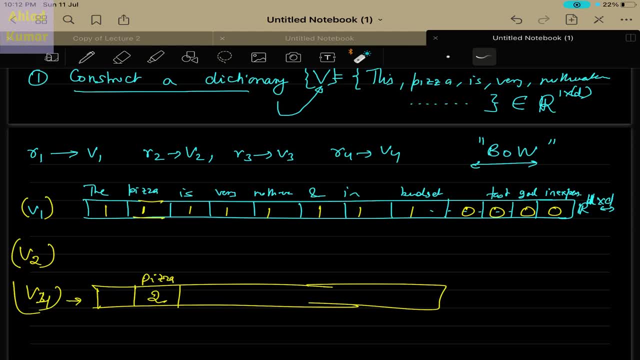 So one of the disadvantages of, you know, representing the reviews in the form of a vector representation here is that is the length of this vector. So you can see the length of this vector. can, you know, run to a very large value if your data corpus contains, you know, large number of reviews. 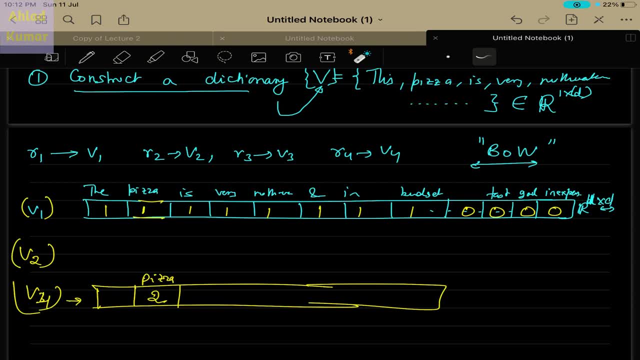 So, for example, if you have any practical data set of Google, which has large number of reviews, what will happen is the amount of words that are used in these reviews will increase tremendously. So the value of D will be very large. So the value of D here will be very large. 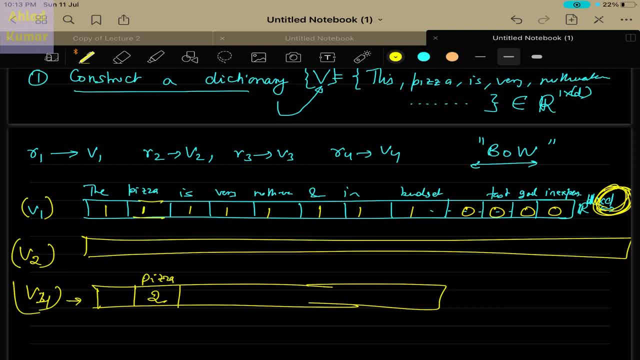 So what happens is, you know, if the value of D is very large, let us say if the value of D is 1000, so only few of these entries in this vector will be ones, and the rest of the remaining elements of these vector will be all zeroes. 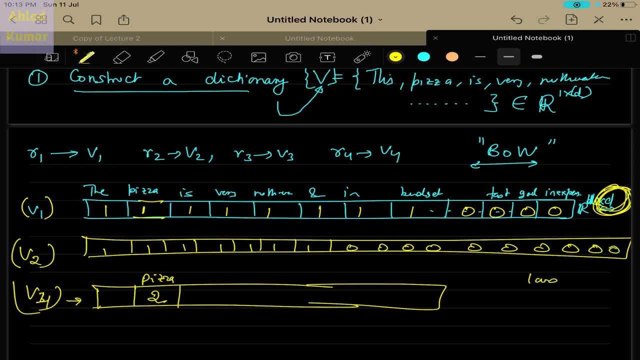 So, out of you know, 1000 entries, only few entries of, let us say, 5 or 10 are 1, but the rest of them are all zeroes. So these vectors, which are actually, you know, created using bag of word algorithms, are actually known as sparse vectors. 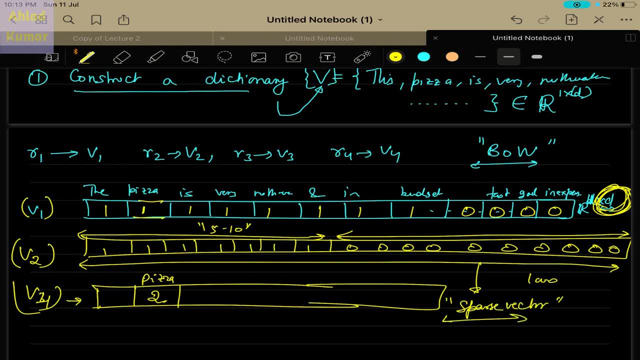 By saying sparse means that only few of them are zeroes. So only few elements of these vectors are 1, whereas the majority of the elements on these vectors are all zeroes. So the sparsity of these vectors is a problem because unnecessarily it will consume a large amount of space because you know, the vector size is very large. 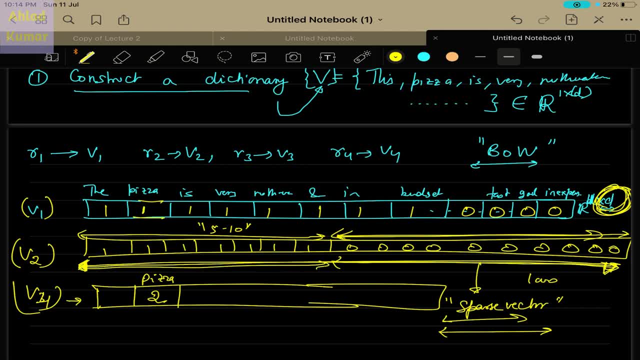 and most of them are zero and few of them are only 1.. So it is a very inefficient way of representing the reviews because of this sparse nature of these vectors. So this is actually one of the drawbacks for this particular, you know, bag of words. 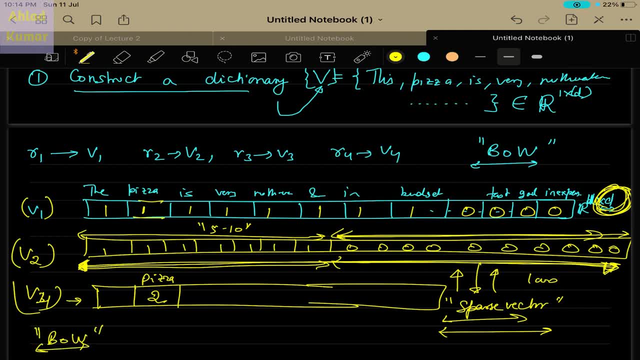 Another drawback that we have in case of representing the vectors using bag of words is that it cannot actually measure the semantic relationship between the reviews. What I am trying to say here is that the vectors that you are getting using bag of word algorithm cannot capture the semantic relationship between the reviews. 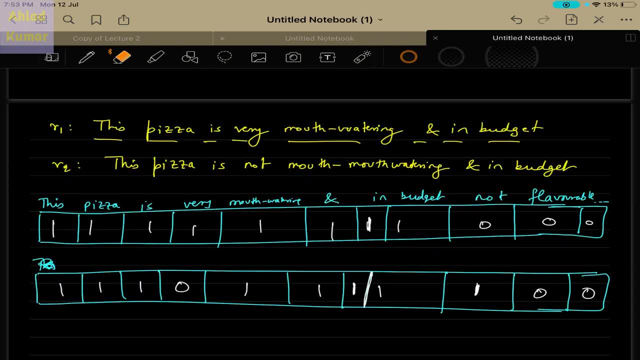 So let us see why this is so. So, in order to illustrate this, I have repeated these- you know, tweets or reviews again here, which we were actually discussing In our earlier slide. So let us see, like you know, let us read these reviews: R1 and R2.. 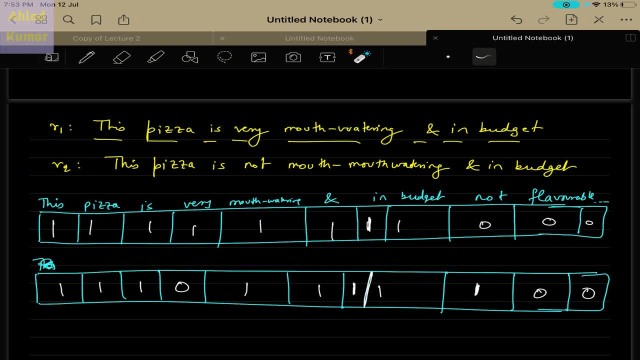 So the first review says that this pizza is very mouthwatering and in budget And the second review says that the pizza is not mouthwatering and in budget. So you can see that both the reviews are, you know, some way or the other. like you know, one is a positive review about the pizza and another one is the negative review about the pizza, but they mutually agree on budget. 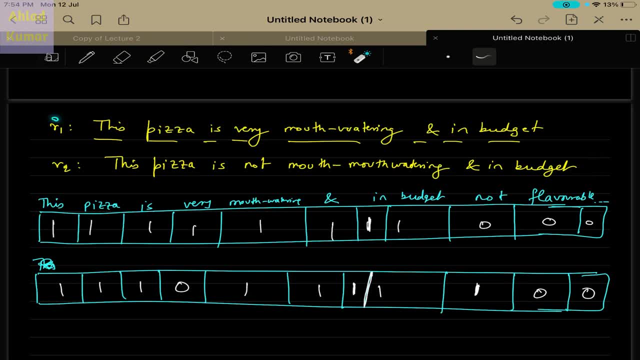 So the important thing is when you convert these reviews into the vector format. So we want to see whether the vectors which are representing these reviews are they capturing the semantic relationship within these reviews or not. So the first review which is here, review R1. if we represent it in a vector format, it looks like this: 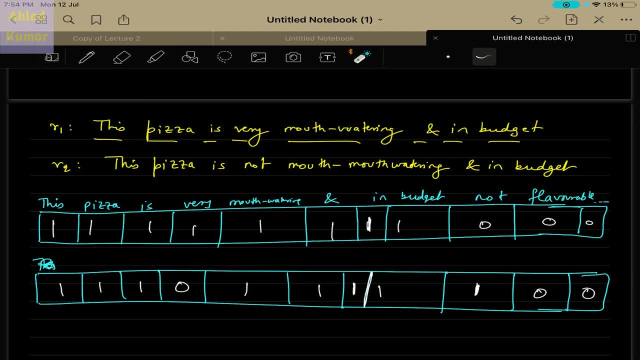 So here you can see the dimension of this vector will be, you know, 1 cross D, where D is the number of words that are present in the total corpus which you are actually, you know, dealing with. So here you know if the corpus has, let us say, 1000 words. 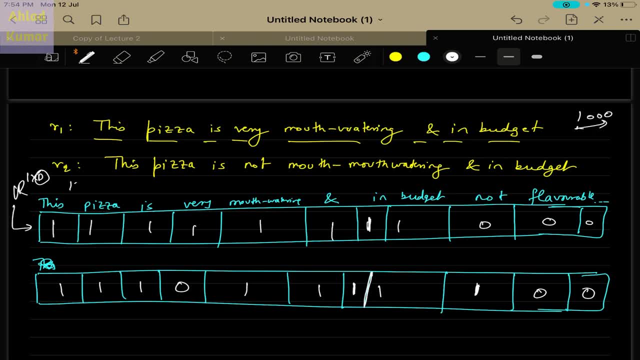 So the dimension of this vector, the one which we are having here, will be 1 cross 1000.. And you can see that the words which are actually present in this review, I am keeping the values corresponding to the presence of that word as 1.. 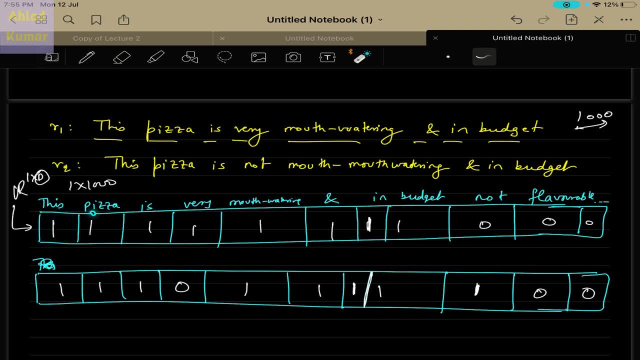 So you can see here, this is present in review R1.. 1 is, you know, pizza is present in review R1.. So I am keeping it as 1 and similarly for other words, also the ones which are present in the review, I am keeping it as 1, but for the rest I am keeping it as 0.. 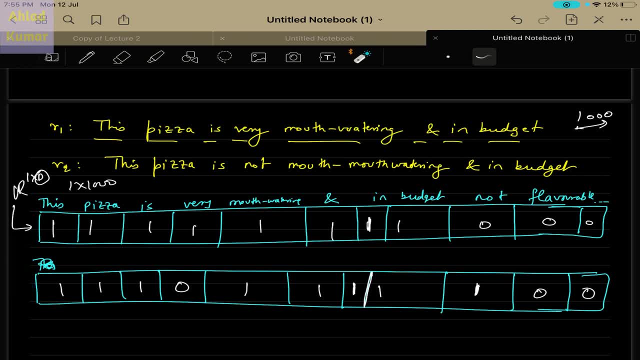 And similarly for the second review also, we wrote this vector where the presence of ones are actually the presence of words in the review and absence of one is basically the absence of word in the reviews. So here we have another vector. So the important thing now is like, if I want to calculate the magnitude of these vectors individually, 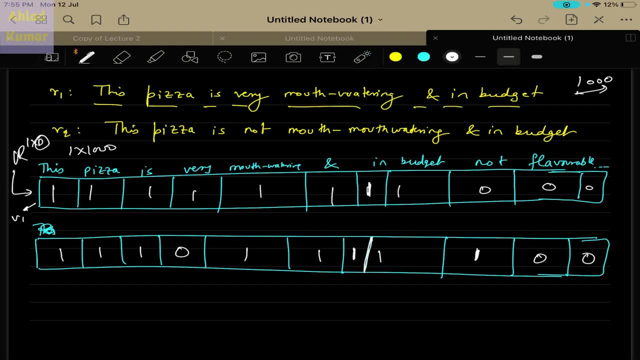 So let me write this vector as, let us say, V1 and this vector as V2.. So if I calculate the magnitude of the vectors V1 and magnitude of the vectors V2, then it will be what it will be under root of 8, and for V2 also, it will be under root of 8.. 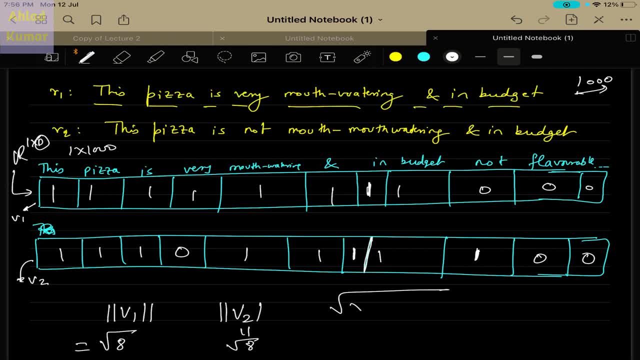 So you can calculate that. it is very easy. You know each of the components. you have to square and then take the square root and these x1, x2, x3 are all x1, x2, x3. all of them are the individual components of these vectors. 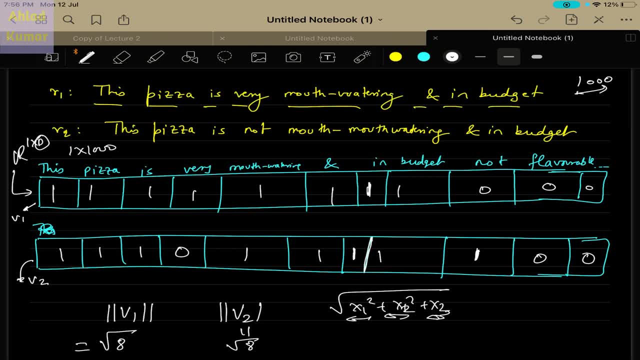 So if you take square root of under 8, it is something around, you know, 2.82 and same for this. So these two vectors, though they have same vector length, but the important thing is you know to calculate how much far these two vectors are in the d dimensional space. 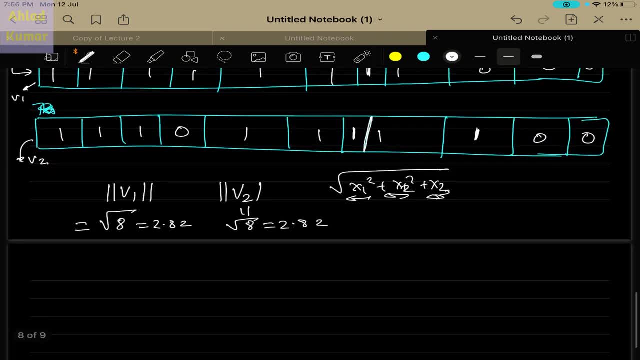 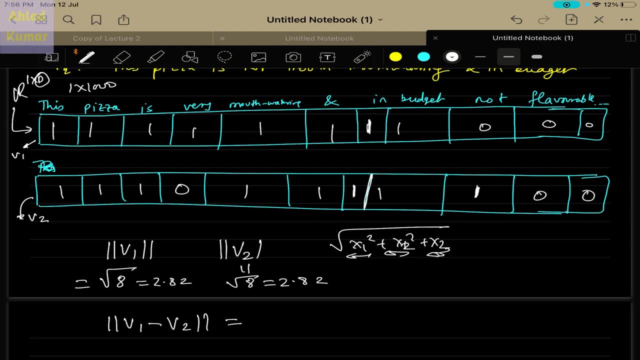 That is one of the important things. So if we calculate the distance between the two vectors, V1 and V2, then the distance between the two vectors comes out to be square root of 2.. That is very simple. This is just if you observe it here. this subtraction cancels out. this subtraction cancels out. only element of the vector which remains is this and this: 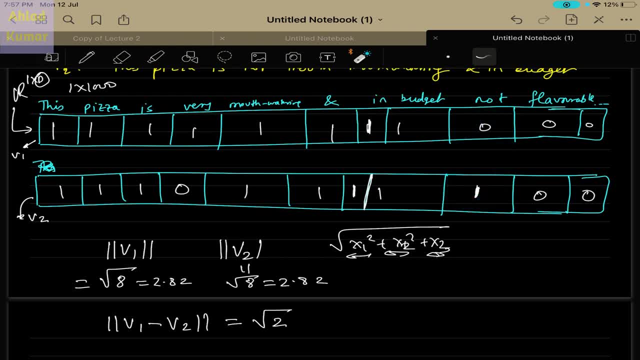 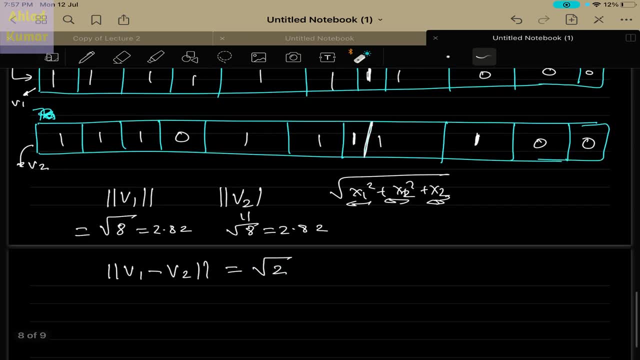 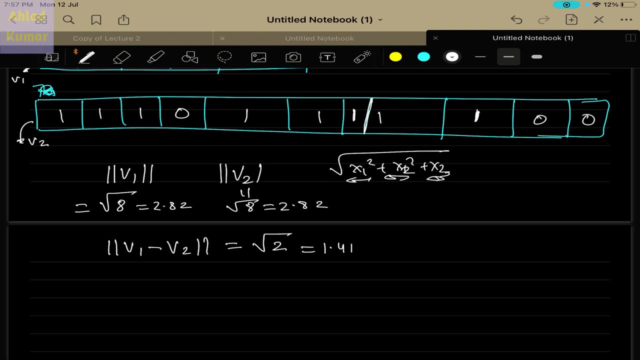 So the number of words which are actually differing in the two reviews contribute to the difference Difference in the vectors. So here we have this value as root 2.. So now you observe carefully that you know the distance between the two vectors, V1 and V2, is only 1.414. 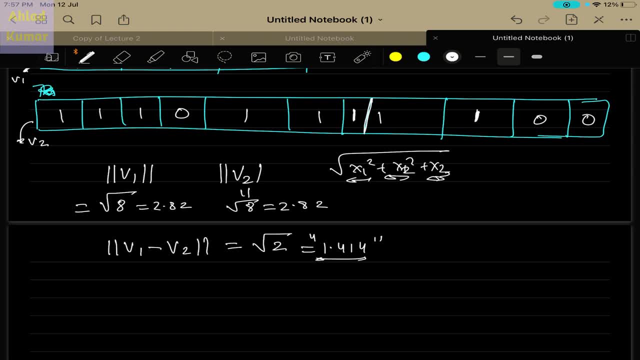 So now you can see that you know the magnitude of the vectors is 2.8 and the difference between these two vectors is 1.414.. So that means you know these two vectors are very close to each other. This is one vector, V1, and another vector is V2.. 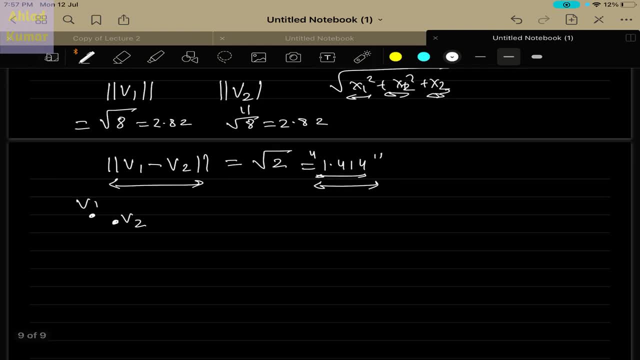 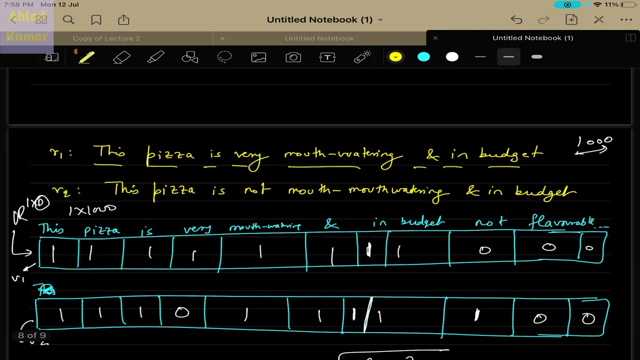 So if they are very close to each other, the tendency is, you know, that the machine learning algorithm will, you know, cluster these two vectors into a single cluster. So this single cluster will be, you know, let us say, positive comments. So the key take away point here is that, using bag of words, the distance between V1 and V2 is very small. but you know, if you observe carefully, the reviews are completely opposite of each other. 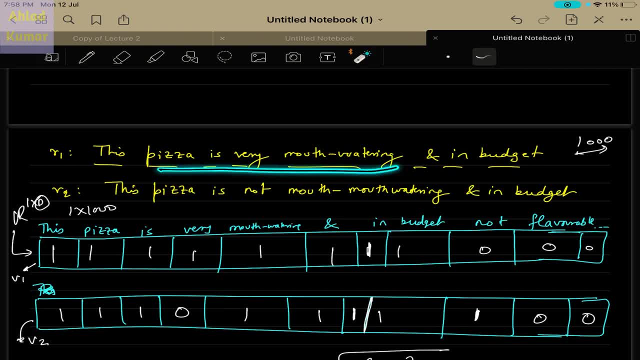 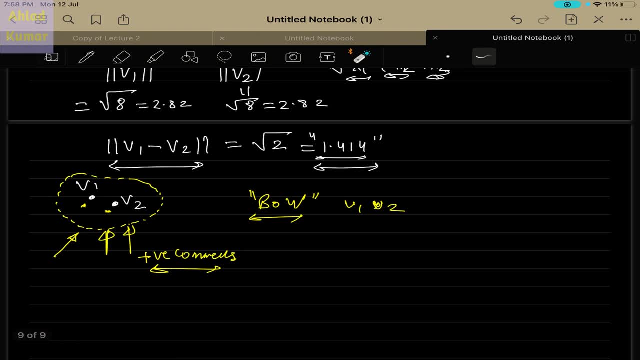 One review is saying that the pizza is very mouthwatering. another review is saying that the pizza is not mouthwatering at all. But what we are doing now we are actually, you know, because the distance is too close. the machine learning algorithm may cluster them into single cluster and it might give it as a positive comment. you know, cluster. 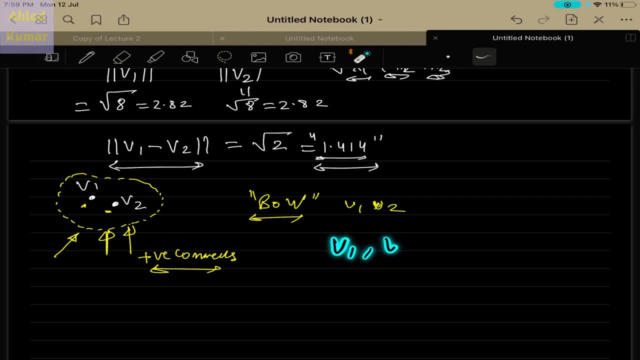 So this means that you know, using these vectors, V1 and V2, using bag of words is a problem Because V1 and V2 are not able to capture the semantic relationship in the reviews. So first review, V1 is positive, but V2 is negative review, but still they are very close towards each other. 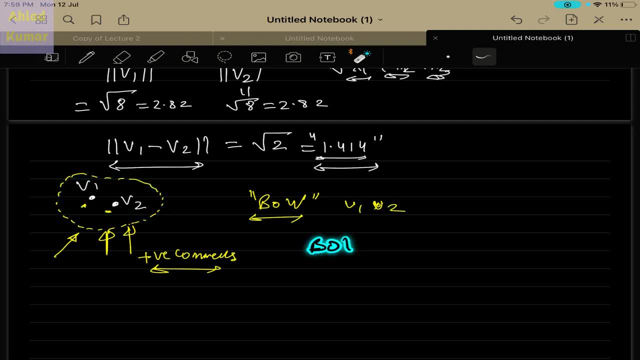 So these are the basic problems that we have in bag of words. The first one is, you know, as we discussed, the sparse nature of the, you know, of the vectors, sparse nature of the vectors, of the vectors Which require a large space to be, you know, used for storage, because, you know, the dimension of the dictionary D can be very large.